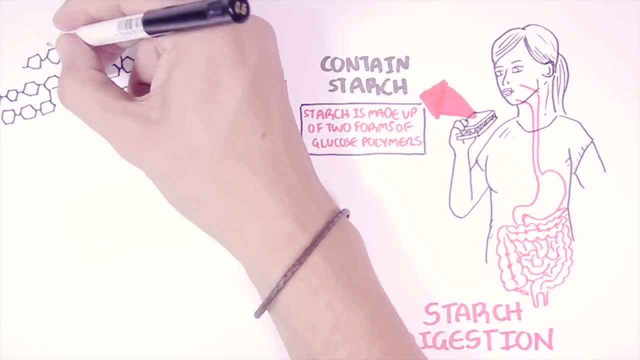 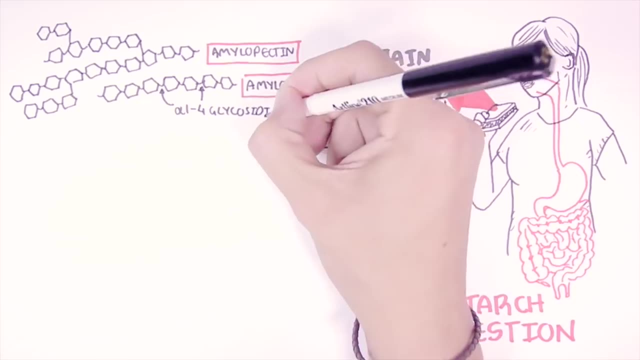 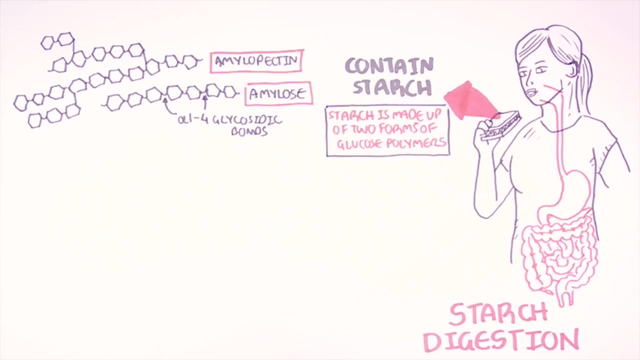 amylose and the branched amylopectin. Amylose is a linear chain of glucose linked together by alpha-124 glycosidic bonds. Amylopectin are linear chains of glucose with branch points creating a tree-like figure. In amylopectin, the 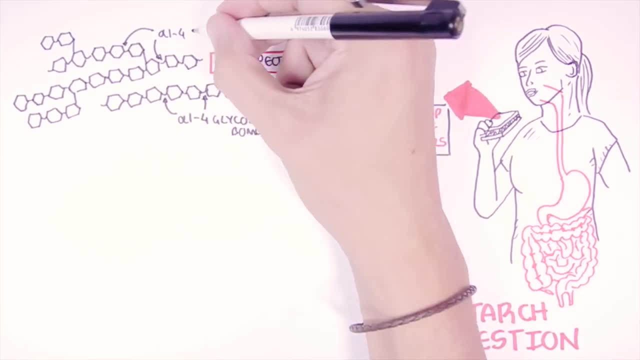 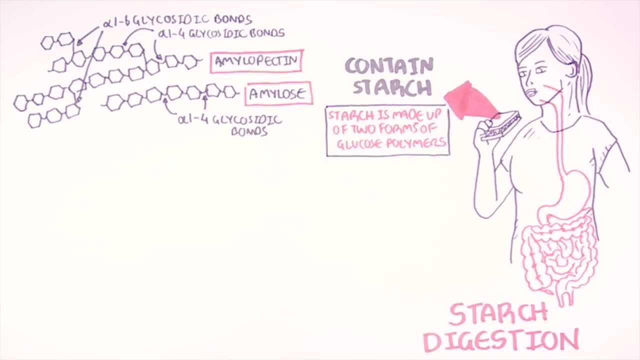 glucose molecules are also linked by alpha-124 glycosidic bonds, but the branch points are linked by alpha-126 glycosidic bonds. So now let's see what happens when starch is ingested. What happens first is that the mouth will break down the starch, both physically and chemically. 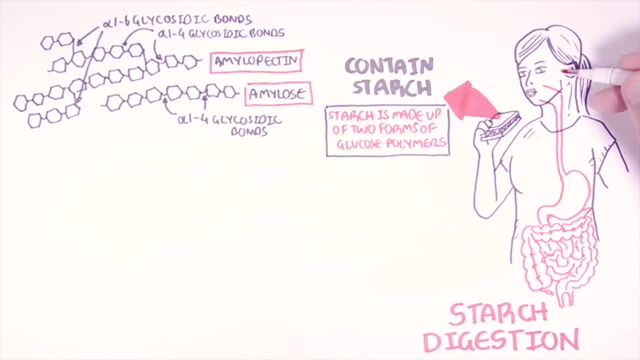 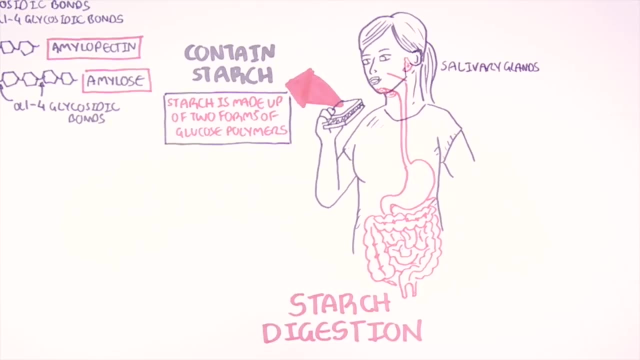 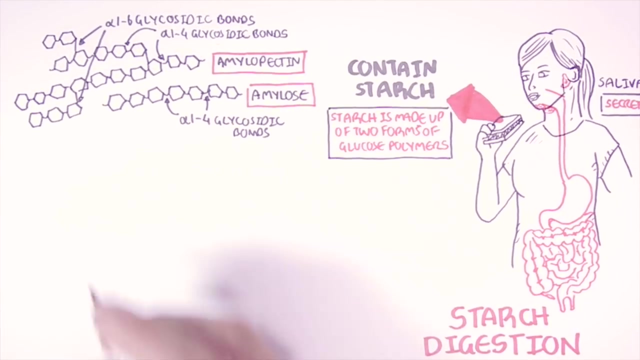 Physically by the jaws, teeth and tongue. chemically by the salivary glands. The salivary glands secrete saliva, but also the enzyme within it called salivary alpha-amylase. What alpha-amylase essentially does is that it will break these bonds. here: the alpha-124 glycosidic. 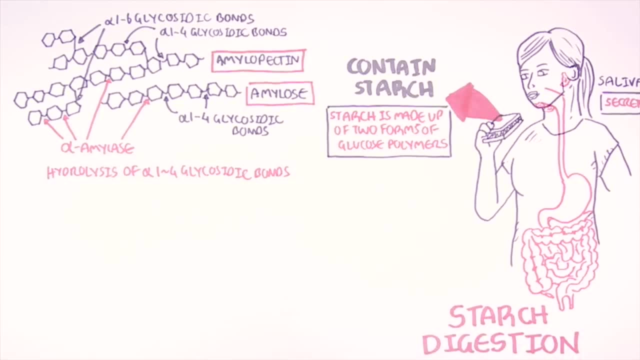 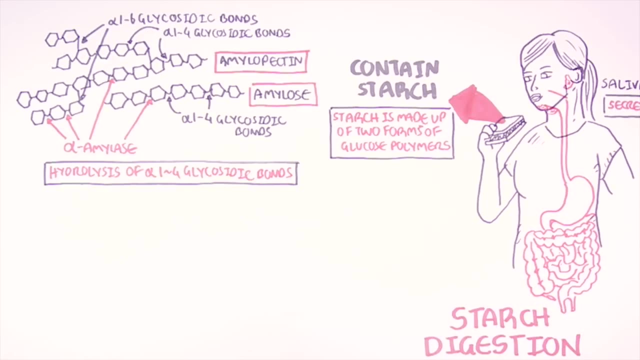 bonds. So alpha-amylase hydrolyzes alpha-124 glycosidic bonds. Hydrolyzing in this respect means breaking down. Amylase will only break down the starch partially and then from the mouth the starch will travel towards the stomach- here Starch. 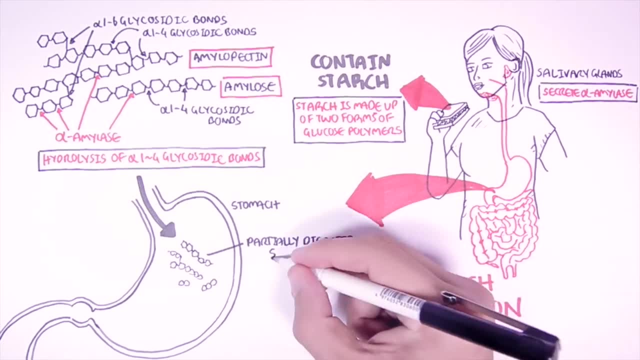 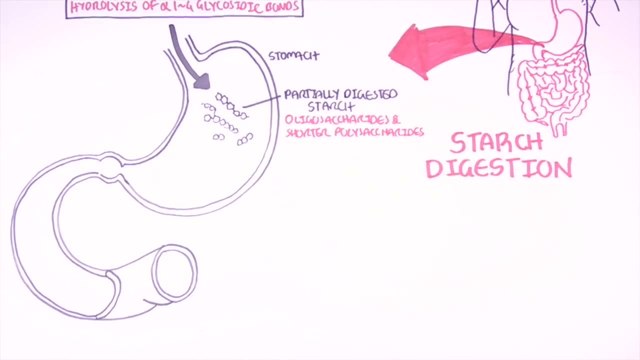 is only partially hydrolyzed into oligosaccharides and shorter polysaccharides. once it reaches the stomach, Starch is only hydrolyzed partially because once the starch comes down to the esophagus, into the stomach, the amylase becomes inactivated. This is 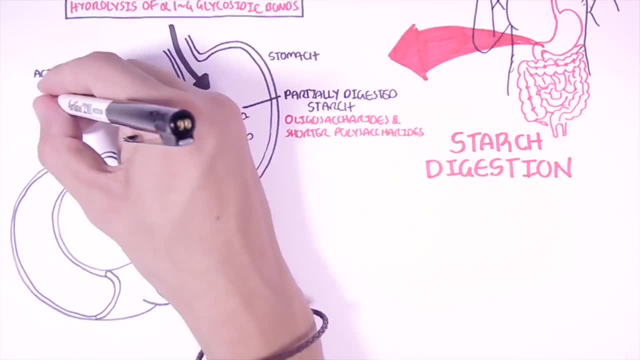 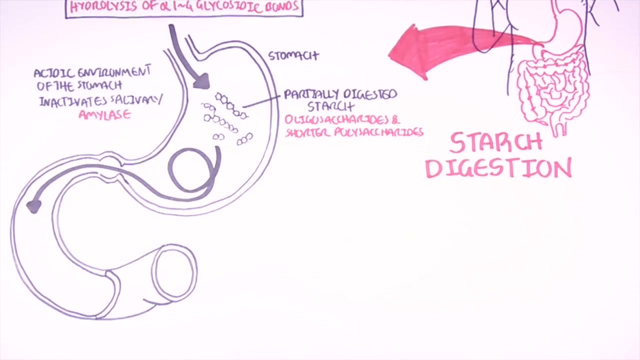 because the acidic environment of the stomach actually inactivates the salivary amylase, and so starch digestion does not occur within the stomach. The stomach will only mix the content around and then allow the starch to reach the small intestine, And it is within the small intestine where most of the digestion and absorption of starch 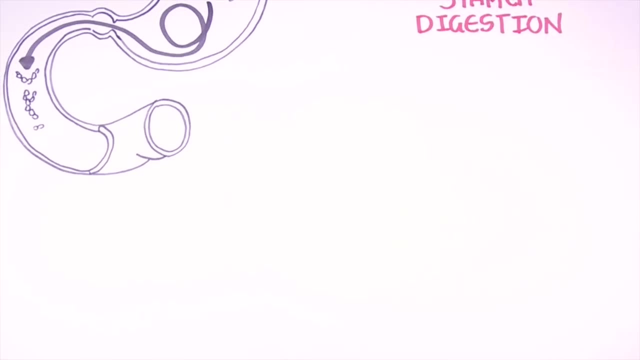 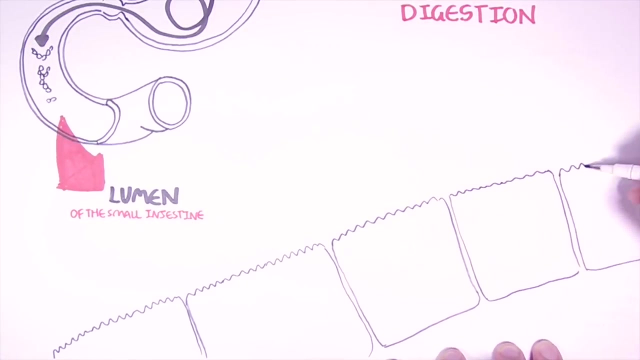 takes place. Let's zoom into the small intestine and see what happens with the starch. So we're zooming into the lumen of the small intestine. Within the lumen of the small intestine we can find the cells, the cells of the intestine, known as enterocytes. The enterocytes are also called 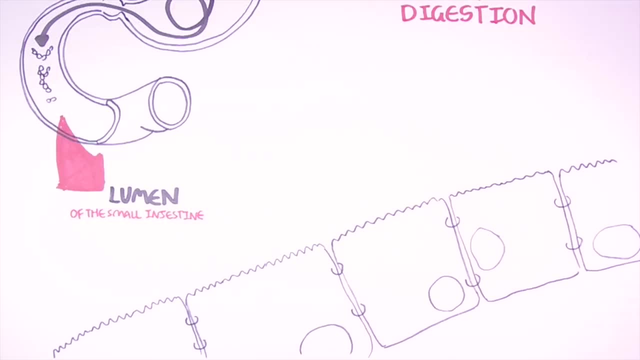 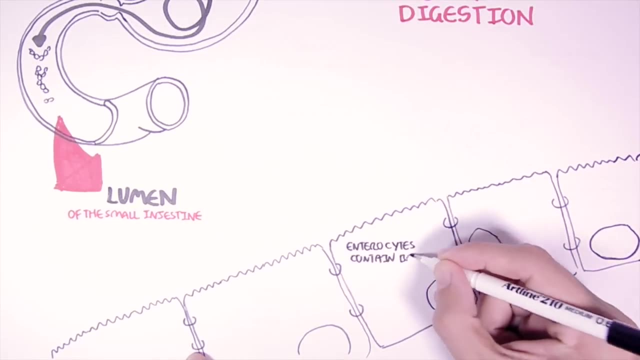 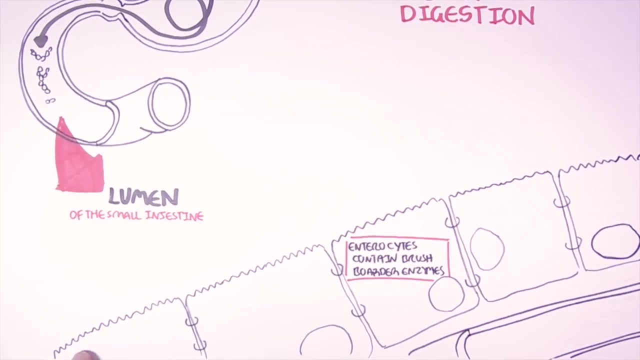 the absorptive cells because they absorb the nutrients. But the enterocytes also contain these enzymes, called brush border enzymes, that play a role in the digestion of starch. Below the enterocytes we have the bloodstream. So when starch reaches the small intestine we're able to find the small intestine. and, as we see here, we're able to find the small intestine. and the small intestine can also be found here, which means that the large intestine, the small intestine, also contains this amount of protein in the small intestine. If this happens, the large intestine, small intestine- it is already in a partially hydrolyzed form. remember Now. when starch reaches the small intestine, another organ known as the pancreas, which is situated here, will begin to secrete alpha amylase. So there was alpha amylase secreted from the salivary glands and the pancreas, The pancreatic. 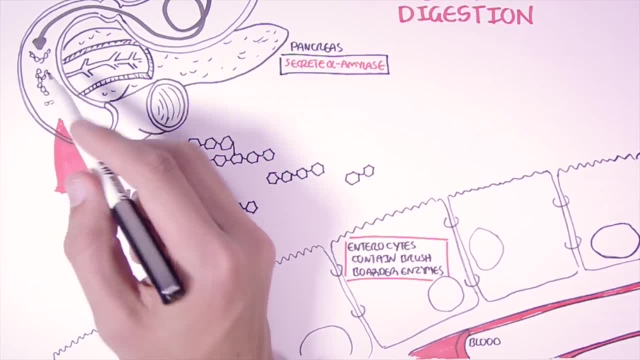 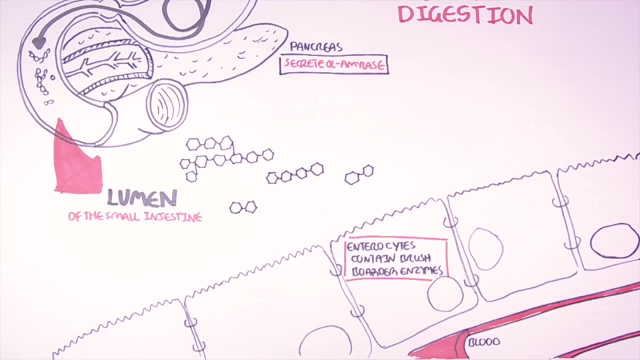 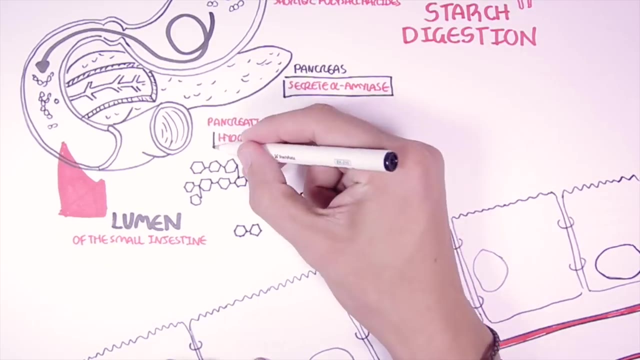 alpha amylase will be secreted into the small intestine, where it will break down the alpha-124 glycosidic bonds, just as what the salivary amylase did. So pancreatic alpha amylase hydrolyzes the alpha-124 glycosidic bonds, breaking down. 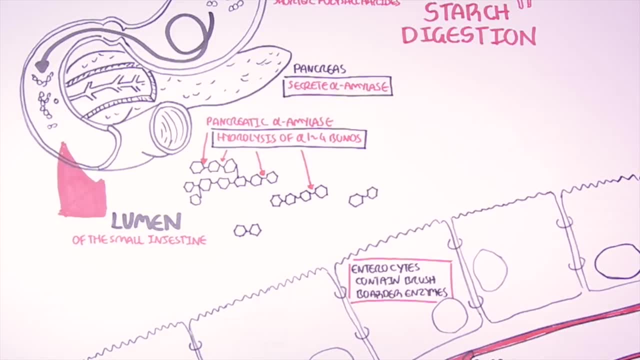 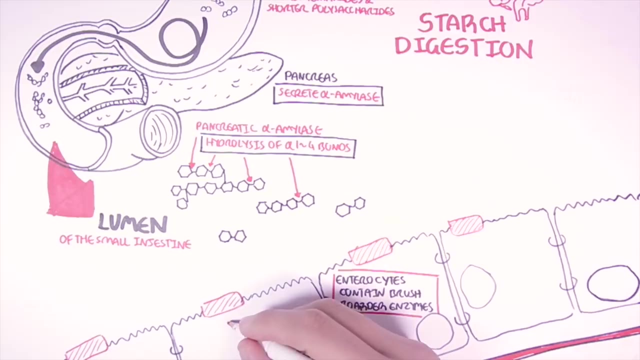 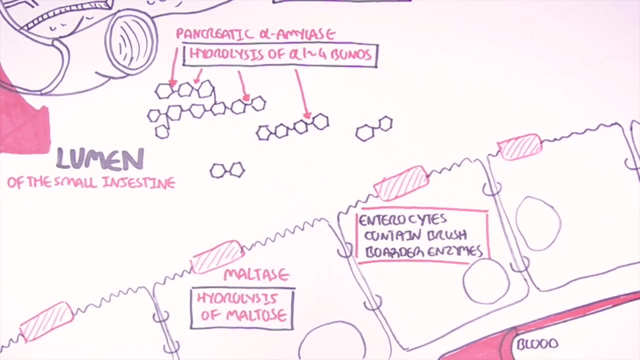 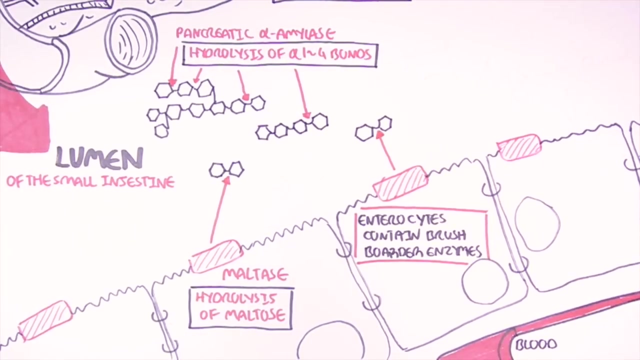 the starch. further, The enterocytes, as I mentioned, also have enzymes called brush border enzymes that participate in the digestion of starch. These enzymes include maltase, which will hydrolyze maltose. Now, maltose is essentially two glucose molecules linked together, So maltase will hydrolyze these. Then you have another. 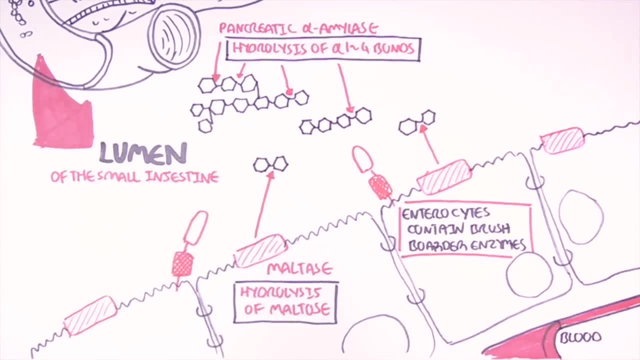 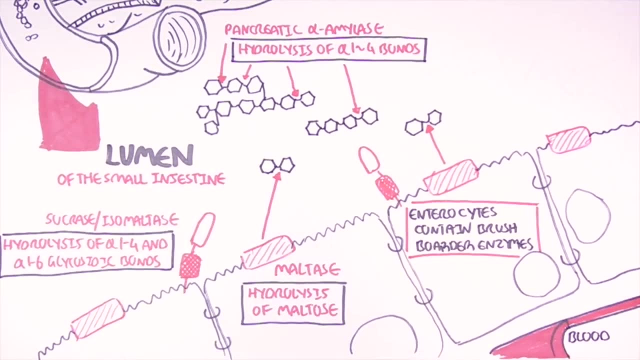 brush border enzyme called sucrase isomaltase. Isomaltase will hydrolyze both the alpha-124 glycosidic bonds and alpha-126 glycosidic bonds. So what is important to know is that isomaltase will hydrolyze. 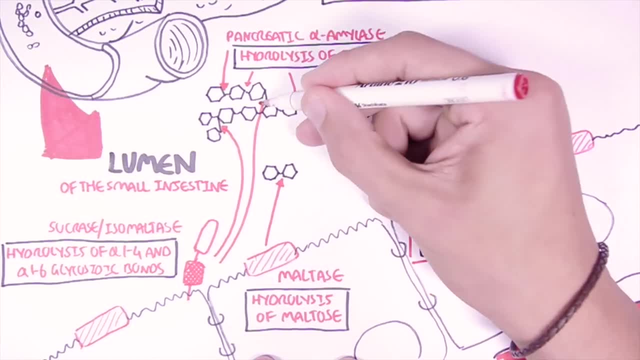 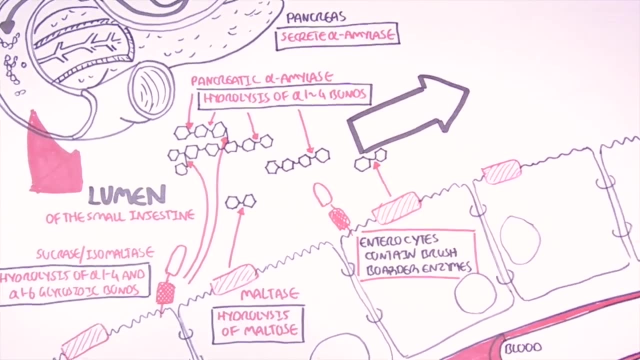 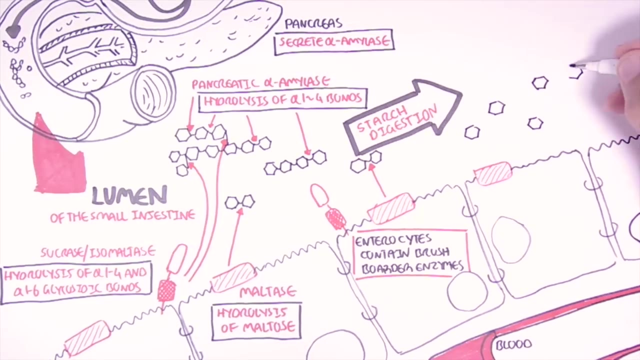 the branch points of starch here. Therefore, starch will encounter all these enzymes in the small intestine and will be digested. It will be broken down into their building blocks. The main reason why starch is so important is that it is the main source of many glucose. 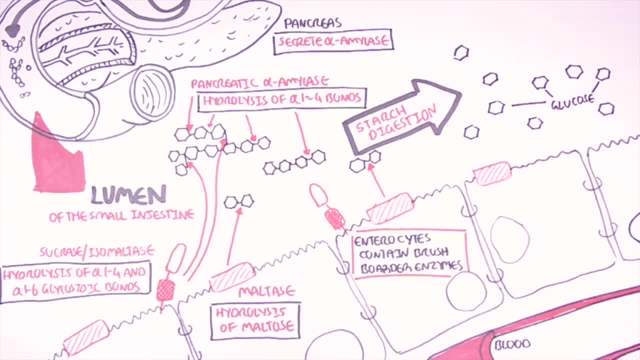 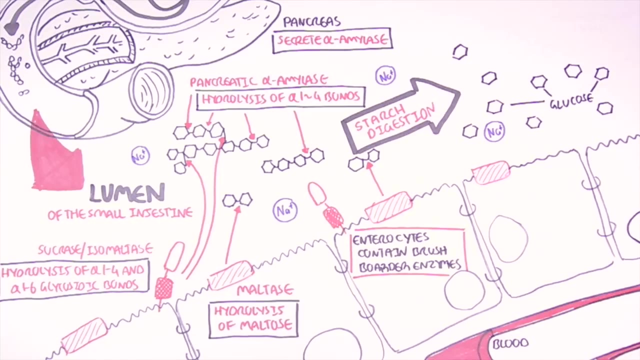 molecules. This means that it contains the main source of many glucose molecules, which is glucose. So through starch digestion we will end up with many glucose molecules. Now, within the lumen of the small intestine, we also have many sodium ions that actually play a critical role in the absorption of glucose into the body. 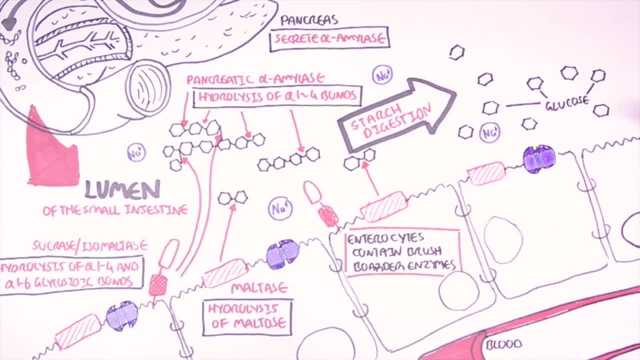 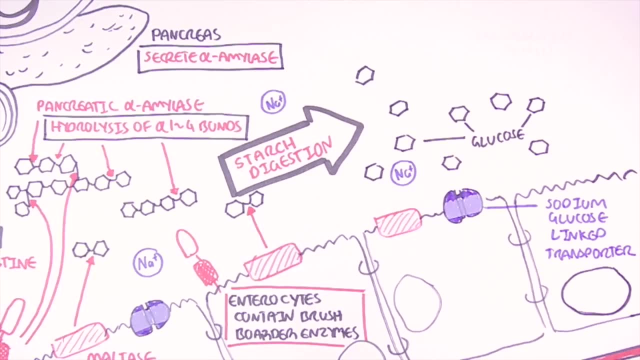 find these transporters called sodium-glucose-linked transporters, or SGLTs. These sodium-glucose-linked transporters are found on the apical surface of the enterocytes, so on the top, And what they do is that they function as a co-transporter for both sodium and glucose. 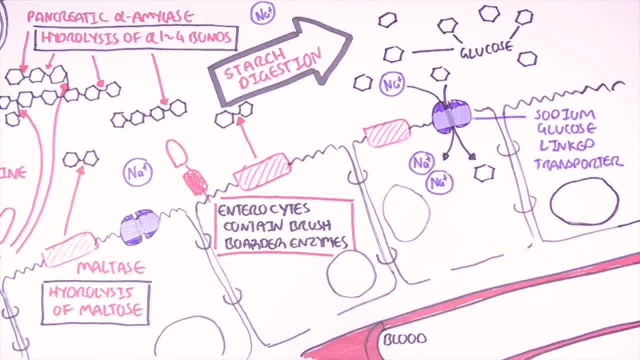 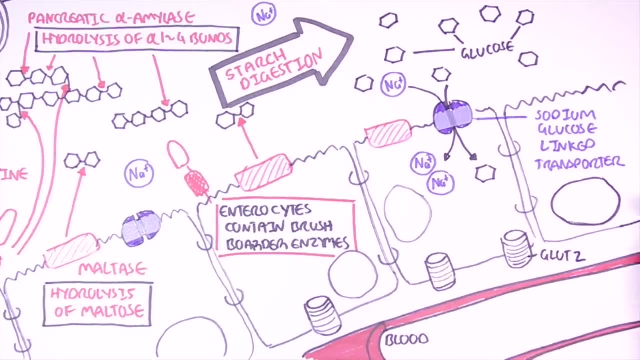 Two sodium ions will enter for one glucose molecule. Once glucose is within the cell, it can be reabsorbed by the bloodstream through a GLUT2 transporter. The GLUT2 transporter is found on the basal surface of the enterocyte. When glucose is in the bloodstream, it will increase blood glucose levels. 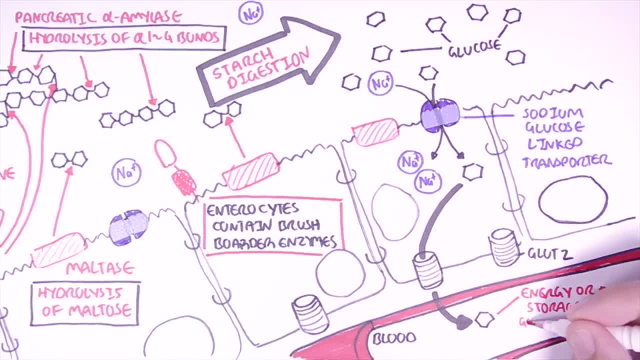 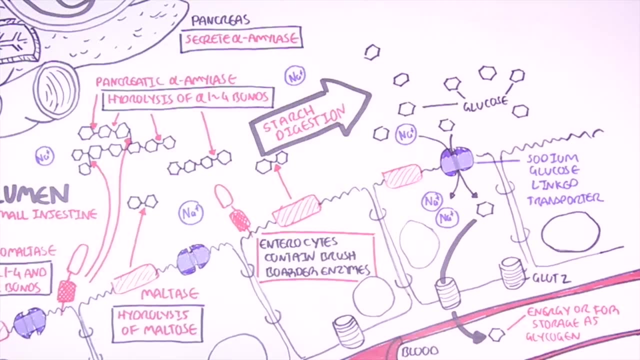 The glucose can be used as energy by tissues or it can be stored away in the liver as glycogen. So glucose is in the bloodstream. So that was the fate of starch. Once it is broken down in the small intestine, it is absorbed by the body and can be used as energy. 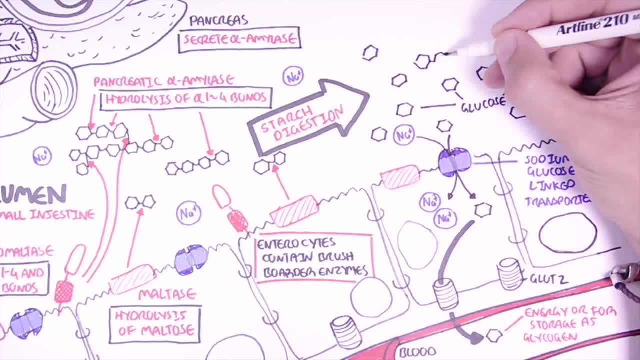 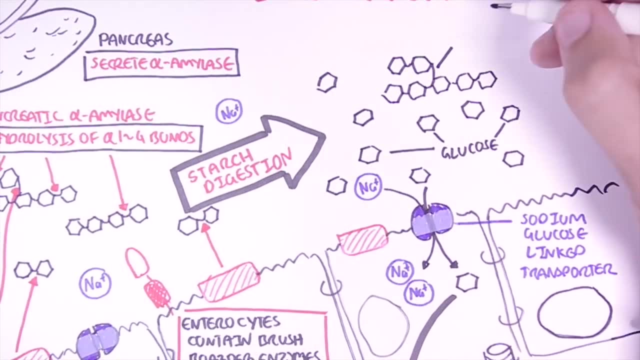 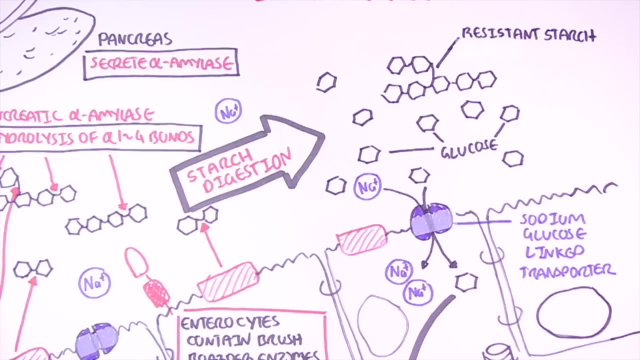 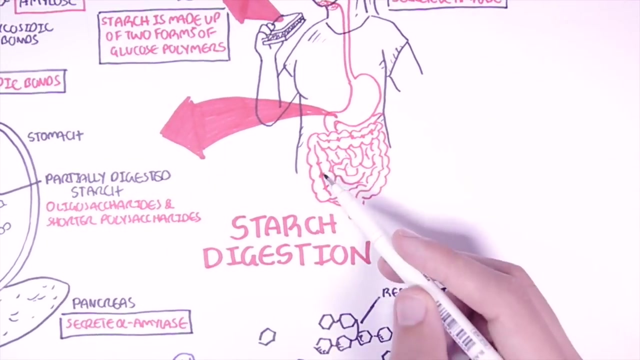 However, not all portions of starch is digested in the small intestine. The portion of starch that resists digestion in the small intestine are known as resistant starch, And this fraction of starch will essentially reach the colon. So what happens to this resistant starch when it reaches the colon? 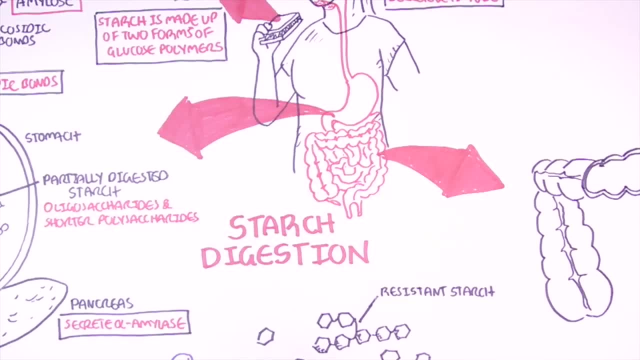 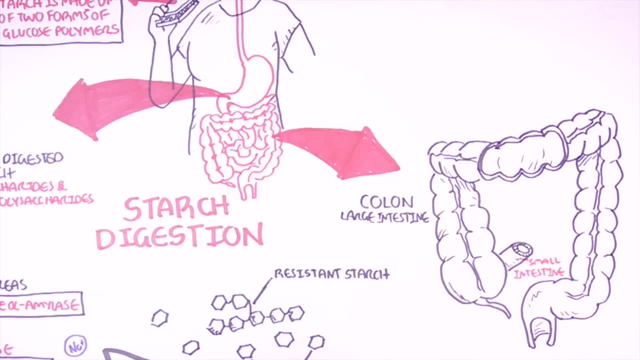 So here we're just zooming into the colon. The colon is also known as the large intestine. The resistant starch will reach the colon after escaping digestion in the small intestine. Now, within the colon, the resistant starch will actually undergo fermentation By the gut microbiota.